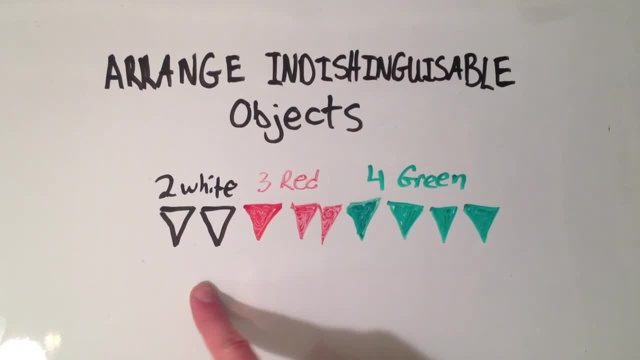 flag and this green flag. it would look exactly the same. So maybe you're a lifeguard or something and you have so many flags And you can only make so many flag symbols like this because some of your flags are the same color. So, normally, normally what we would do is we say: okay, we have nine objects. 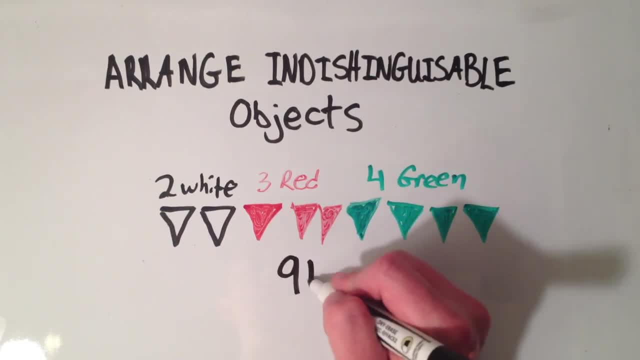 That means there are nine factorial ways to arrange them, Because in the first place you would have nine choices and, to put in the second place, you would have eight choices, and in the third place you would have seven choices and so on, and that was our nine. 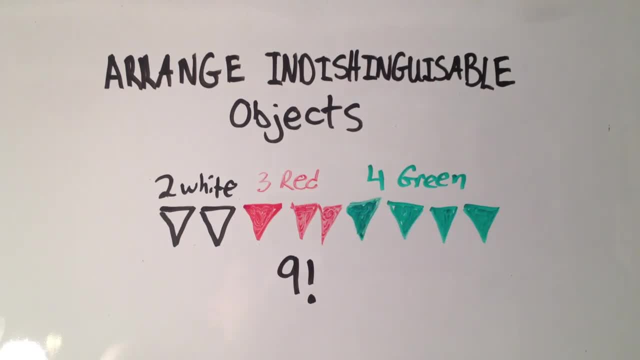 factorial. But that's when the objects were distinguishable, You could tell them apart. So what we do now is we divide by the number of indistinguishable objects. So I see that I have two white flags that are indistinguishable, So I'm going to divide by two factorial. So 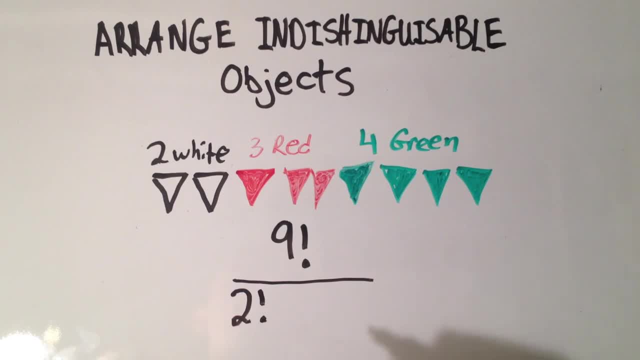 I'm going to divide by two factorial And there are three red flags that are indistinguishable, So I'm going to divide by another three factorial And you can see where this is going. I have four green flags that are indistinguishable. So I'm dividing by four factorial And that 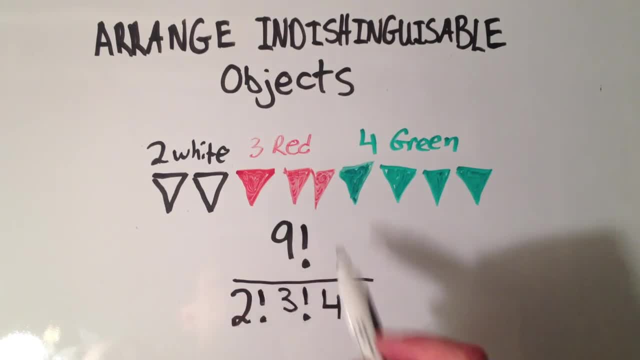 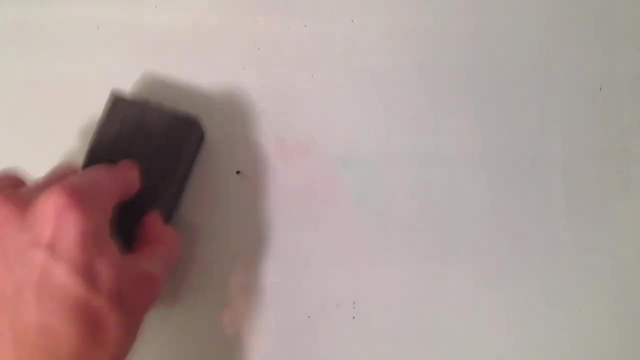 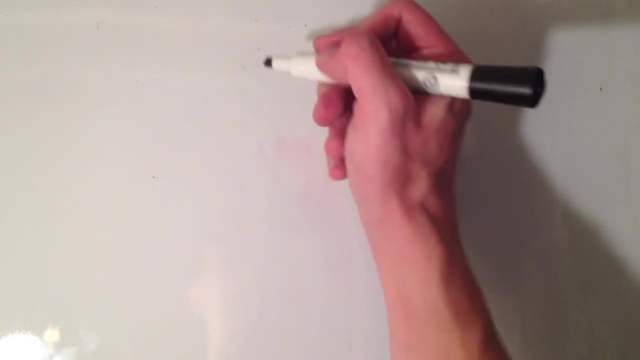 would be your answer, And I'm not going to compute this. You could figure that out, But this is often what they're looking for in a math problem. This is what they're looking for in a math problem: a probability class. So, in general, when you have n objects and a certain number of groups, 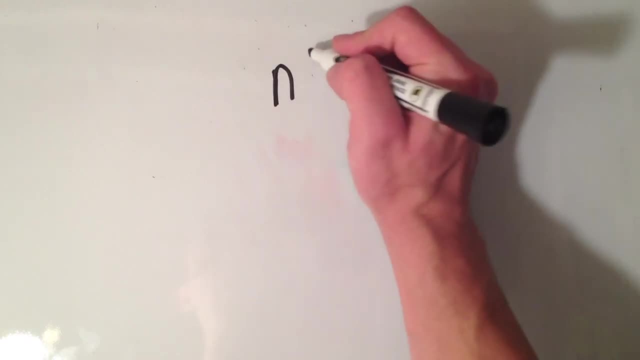 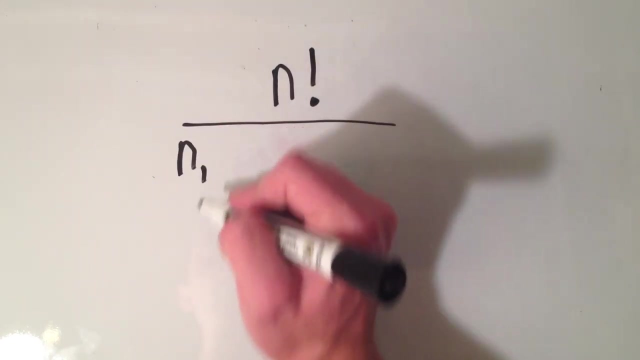 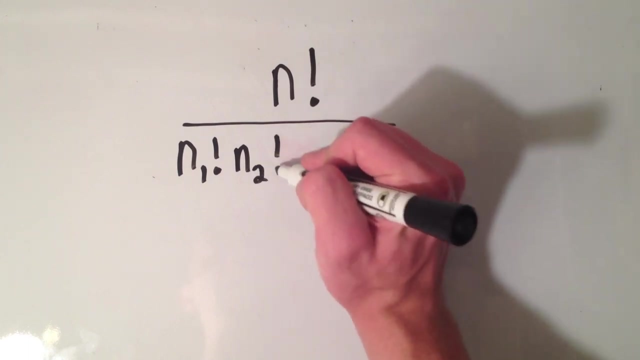 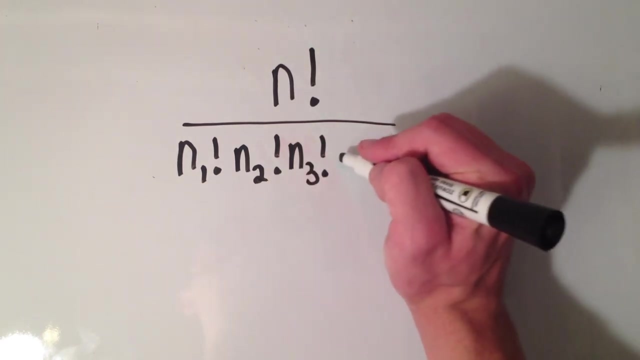 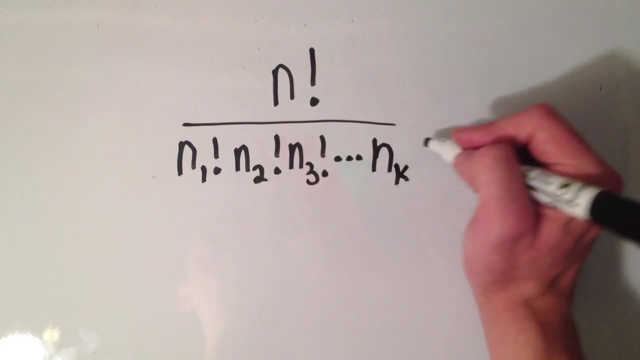 of them are indistinguishable. the formula is: n- factorial divided by however many are in the first group- factorial- times. however many are in the second group- factorial times. how many are in the third group- factorial. and this would go on for however many groups you have that are indistinguishable. Okay, and that's it. I hope you found it helpful.